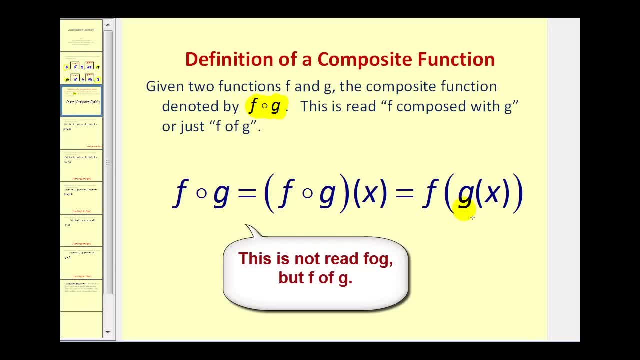 equivalent ways to represent a composition of functions. Remember, for a composite function, the order in which we compose the functions is extremely important. Therefore, when we're given a composite function, we're going to rewrite it in this form here, Because this tells us that we're going to first evaluate function g at the 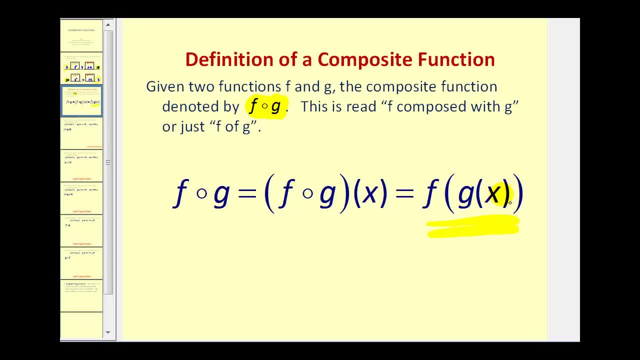 value of x, and the output of that will be the input into function g. So we're going to evaluate function g first and then function f. If the composition of functions is written in this way- And that's almost in the opposite direction that you might think, Notice the f comes before the g. but when it comes to 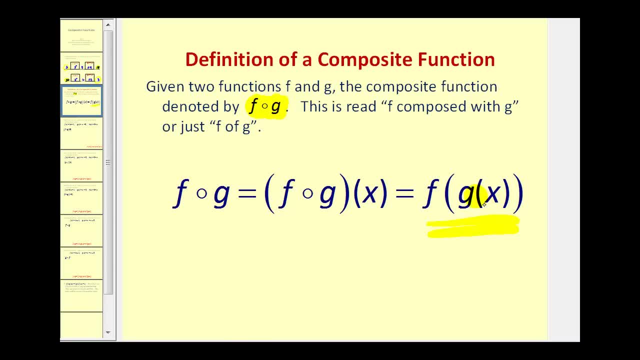 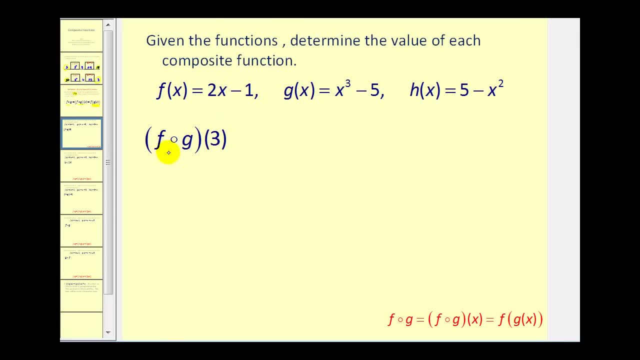 evaluating the given value of x will first be the input into g And that output will become the input into f. Let's go and look at some examples. If we want to evaluate f of g of three, this is going to be equal to f. 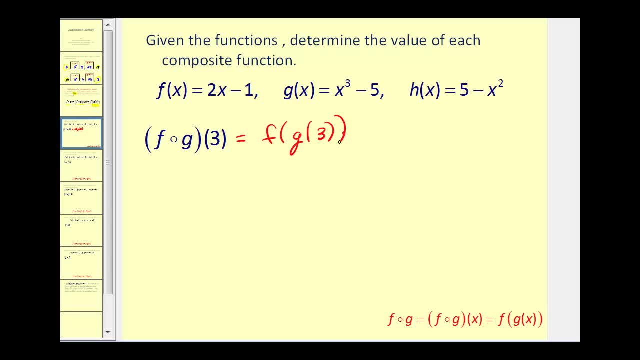 of g of three written this way. And so this tells us that we will find the value of g of three first, and that result will be the input into f. So let's go down here on the side and find g of three. G of three will equal three cubed. 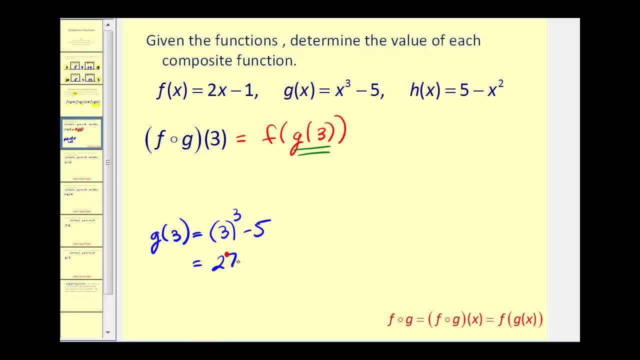 minus five, That will be twenty seven minus five, which is equal to twenty two. Since g of three is equal to twenty two, this just becomes f of twenty two. We found g of three and it was equal to twenty two. Now twenty two will become the. 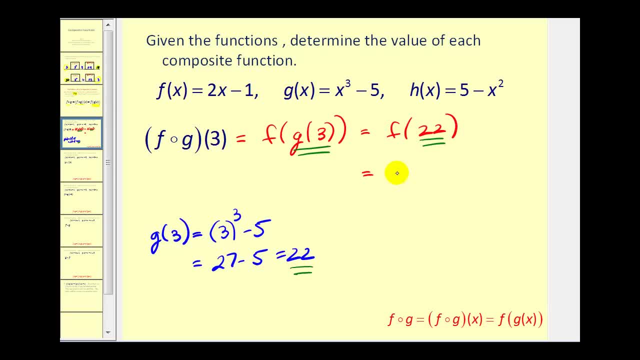 input into f. Notice here f multiplies the input by two and then subtracts one, So we have forty four minus one, So we have forty three. So f of g of three is equal to forty three. Let's go and take a look at another one. Notice this question has the same input. 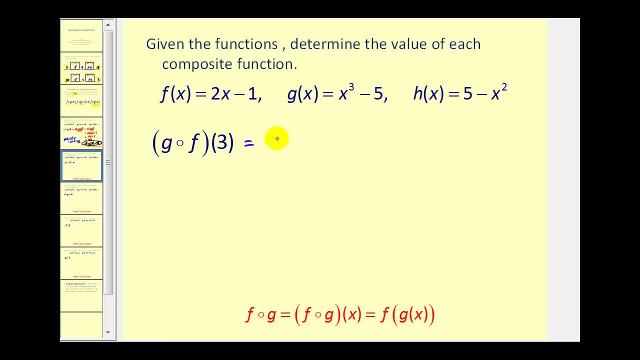 but now instead of f of g, it's g of f. So this is equal to g of f of three. So now we're going to find f of three. first. Let's go down here and do that. F of three is equal to two times x minus one, or two times three minus one. 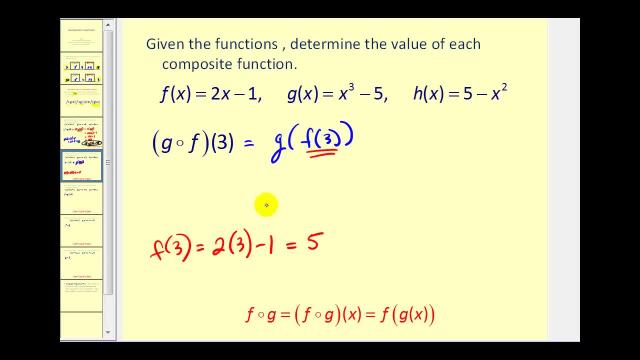 That'll be six minus one or five. So f of three is equal to five. So we can replace this with five. So this becomes g of five, And g of x is equal to x cubed minus five. So we'll have five cubed minus five. So that's one twenty five minus five. 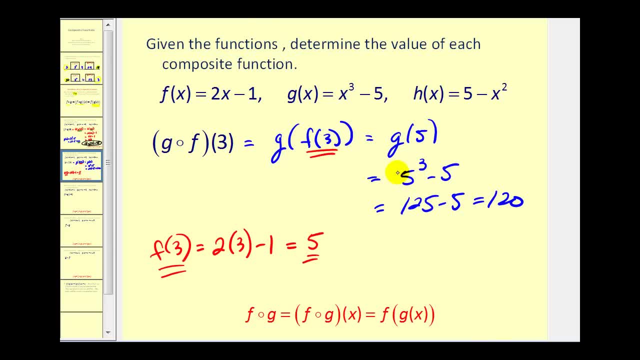 Which is equal to one hundred twenty. So this will be the value of g of f of three. Let's try another. We want h of g of negative one. Well, this is equal to h of g of negative one written this way, And this should key us in to evaluate g of negative one first. So we'll go ahead. 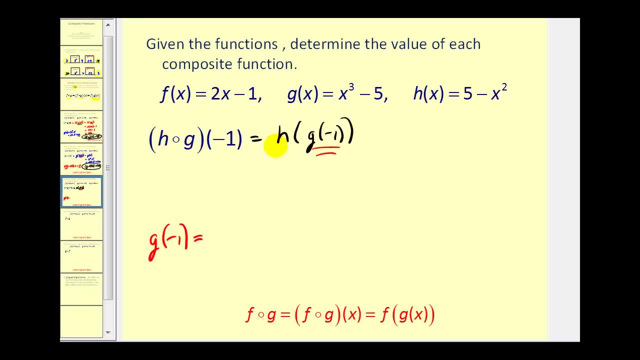 and do this on the side G of negative one. Well, g of x is equal to x cubed minus five. So we have negative one cubed minus five. Well, this will be negative one minus five or negative six. So g of negative one is equal to negative six. So now we can rewrite this as h of negative. 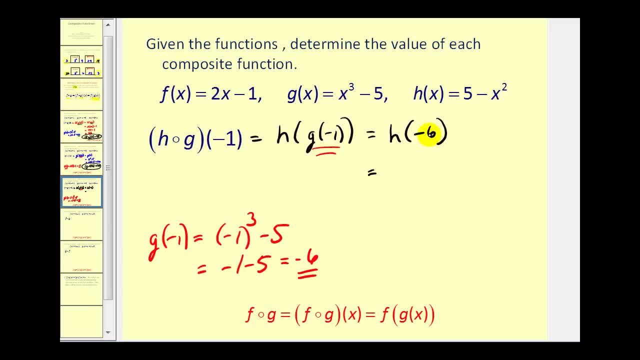 six. So now we replace x with negative six in h. So we'll have five minus negative six squared. Watching our signs, here We're going to have five minus a positive thirty-six, which is equal to negative thirty-one. So h of g of negative one is equal to negative thirty-one. 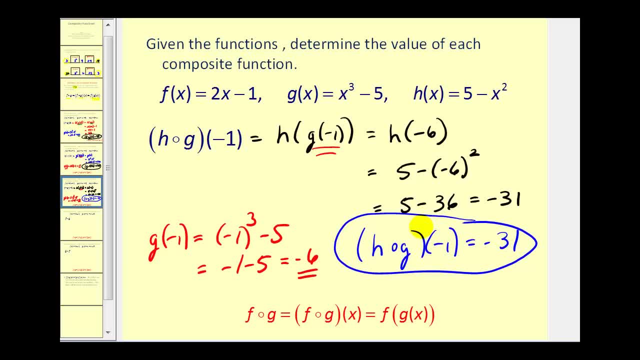 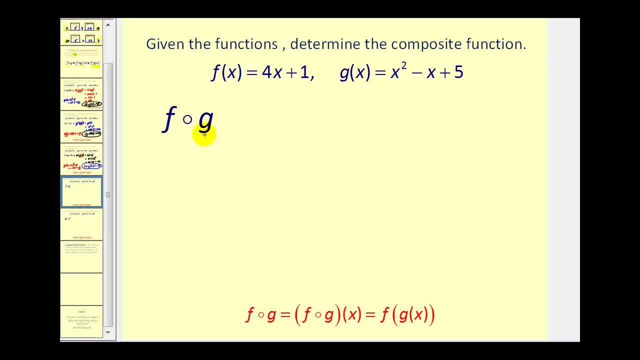 Ok, now there's one other type of problem. we need to look at Notice on this problem. they don't give us an initial input, So what we're going to have to do is input one of the functions into the other function And again, it's important that we follow the correct order. So remember. 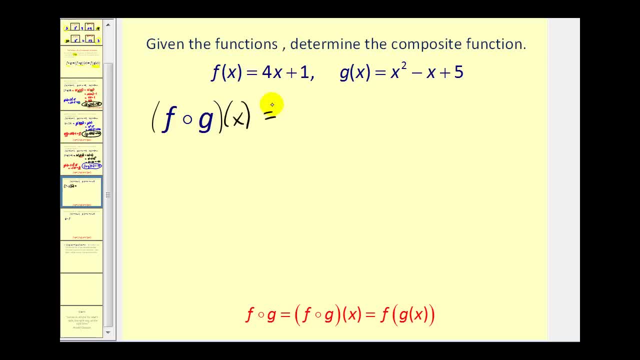 this is the same as f of g of x, Which by definition is equal to f of g of x, written this way. Notice there's no x value to input into g. So the only thing we can really do is replace g of x with x squared minus x plus five. So we need to determine f of x squared minus. 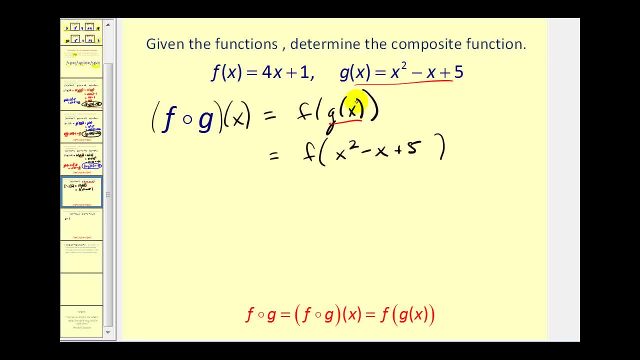 x plus five. So if there's no value to input into g, we have to replace g of x with the entire function. So now, wherever we see an x in f, we'll replace it with this entire expression. So instead of four x plus one, we'll have four times the quantity x squared minus x plus. 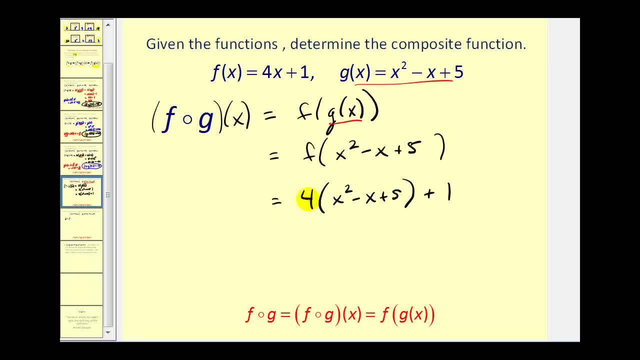 five plus one. So we'll distribute the four And then combine any like terms. So four x squared minus four x, plus twenty plus one. So f of g is equal to four x squared minus four x, and we'd have plus twenty one Sometimes. 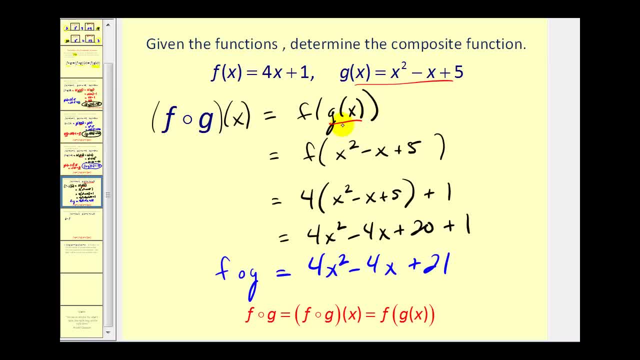 these are a little tricky when you first do these, But the process is exactly the same, except instead of having a numerical value, you have to substitute an entire function into the other function. Let's try one more of these Now. we have g of f instead of f of g, So this is equal to. 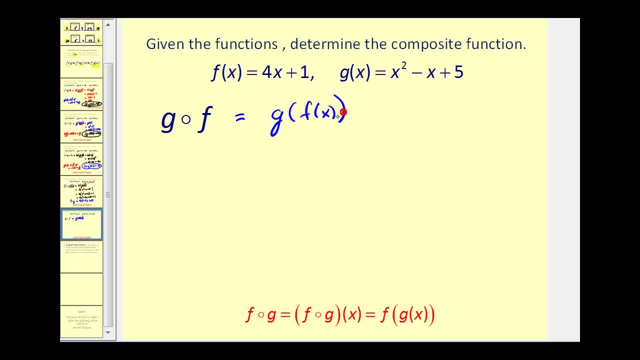 g of f of x. Again, we don't have an input to put into function f, So we're going to rewrite this as g of well. f of x is equal to four x plus one, So wherever we see an x in g, we'll replace it with four x plus one. So we're going to have, instead of x, squared. 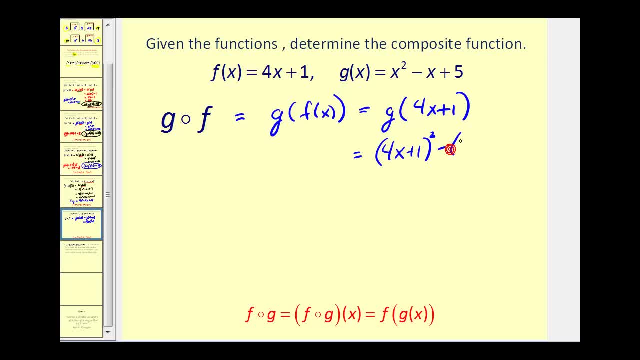 squared minus four x plus one plus five. Here we got the square: four x plus one. There's no shortcuts here. We're going to have four x plus one times four x plus one. This will be minus four x minus one plus five. 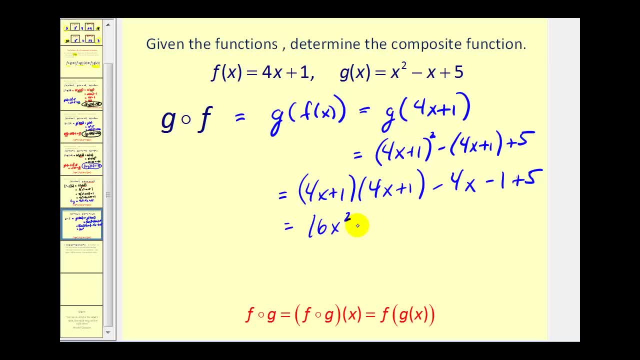 Okay, so we're going to have 16 x squared plus four x plus four x. that's plus eight x plus one minus four x. this would be plus four And one last step and we have one last step. You can see, this type of problem is a lot more work. 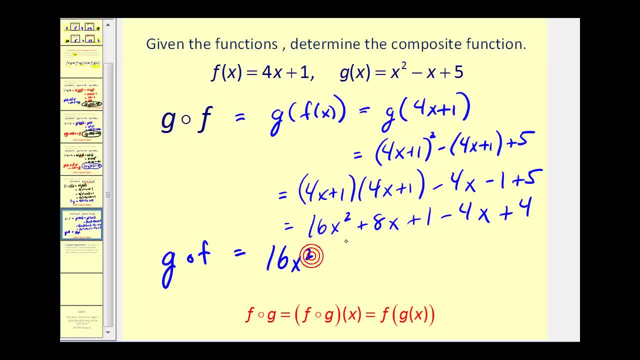 We're going to have 16 x squared plus four x. Here we have a positive one and a positive four plus five, And notice that when we change the order of the composition, the result was quite different from what we had on the previous screen. 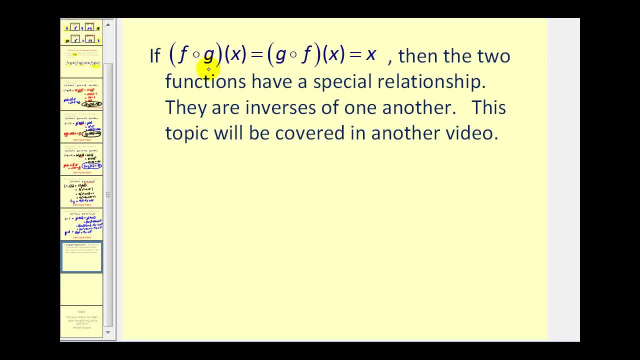 One last comment I'd like to make. If we did determine f of g- and it was equal to g- of f, which was equal to x, then the two functions have a special relationship and they are inverses of one another, And this topic will be covered in another video.